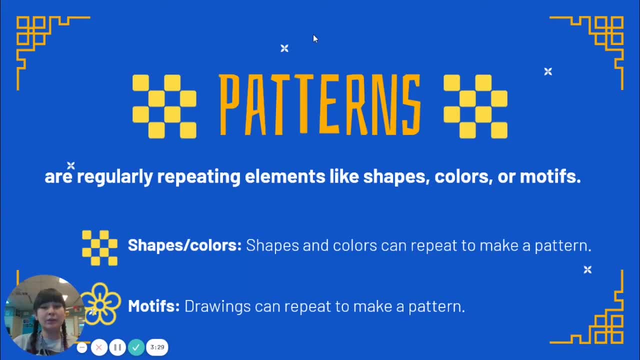 that as well. With this project, we're going to be looking at the principle of design patterns. Patterns are regularly repeating elements such as shapes, colors and motifs. We always talk about the principle of design patterns. We're going to be looking at the principle of design. 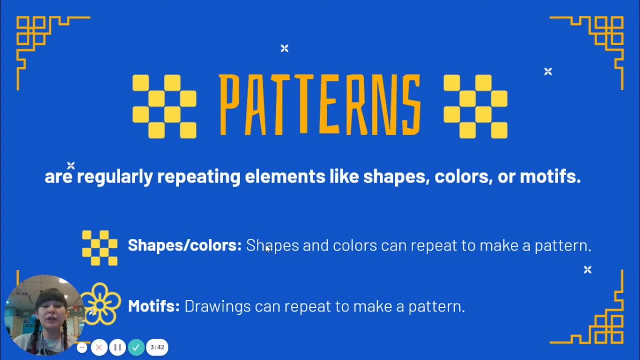 patterns. We always talk about repeating shapes and colors when we do patterns, And when shapes repeat or colors repeat, it can become a pattern. If you have stripes for red and blue, then it would be red, blue, red blue repeating. If you had a pattern with squares and circles, it might. 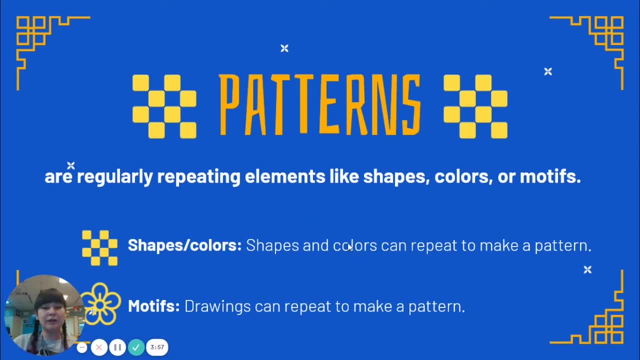 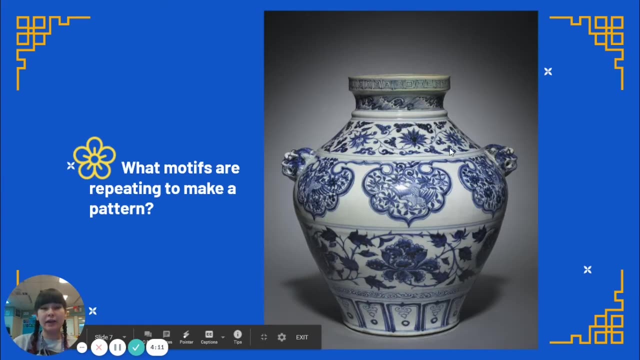 repeat square, circle, square, circle, And that is a pattern that we have talked about. Patterns can also be made with motifs. Motifs are little drawings that repeat over and over, So drawings can repeat to make a pattern as well. If we look at this Ming Dynasty vase, you see that the motif of birds are repeating. There's one here. 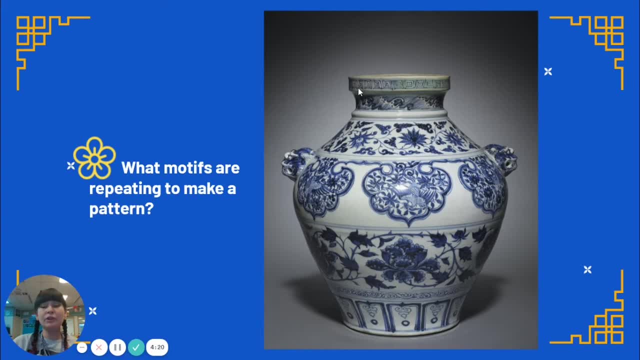 repeats here and repeats here. There are different border designs that repeat. The designs up here are repeating over and over. The waves are repeating. What else do you see that's repeating? You might see vines, flowers repeating more designs. What motifs are repeating in this one? 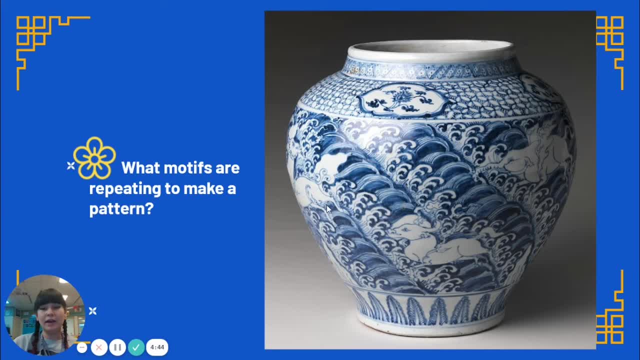 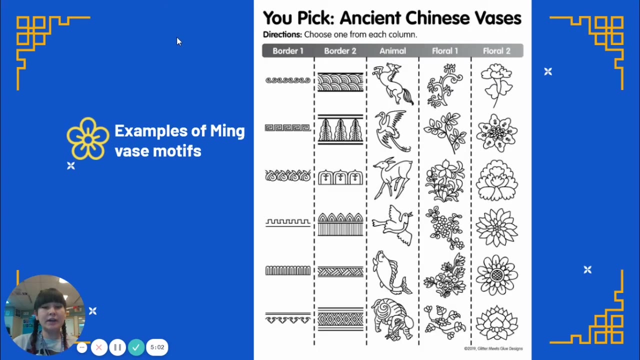 The waves are repeating, The animals are repeating, The flowers and the designs on the bottom are also all repeating And they're all very detailed. Patterns and details are very important part of Ming vases. In this week's assignment I also have a handout that has different types of borders. 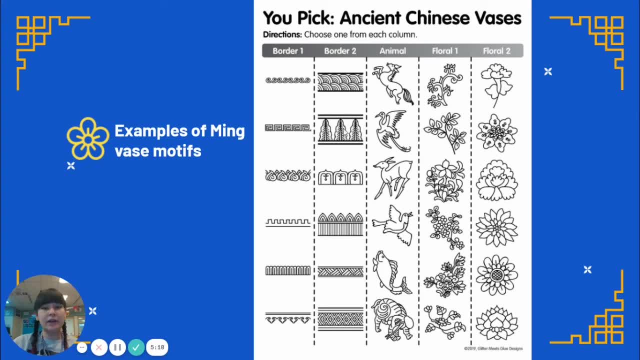 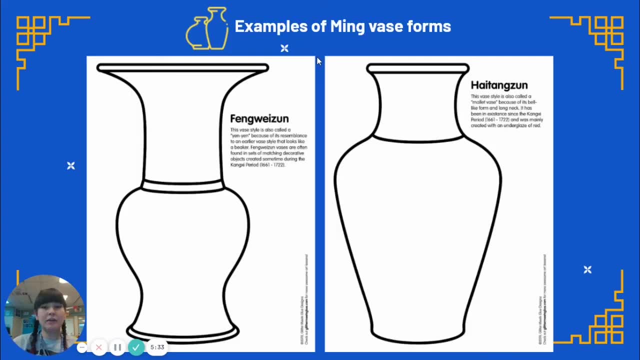 animals and flowers inspired by ancient Chinese vases. So we'll be looking at these motifs when we do our designs. Second graders will be designing Ming-style vases and first graders will be designing Ming-style plates. So, especially for second graders, we'll be looking at different forms. 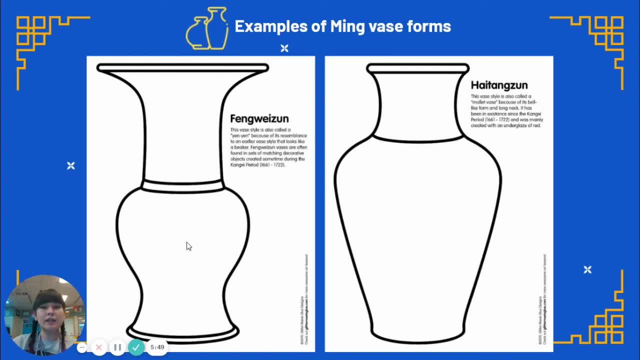 used in Ming vases. Forms are 3D shapes, So if it's flat, like these handouts, it's a shape, but the actual vases that are 3D would be called forms. So there are different kinds of Ming vase.